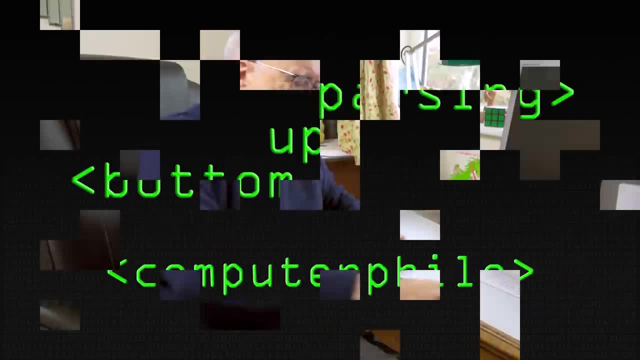 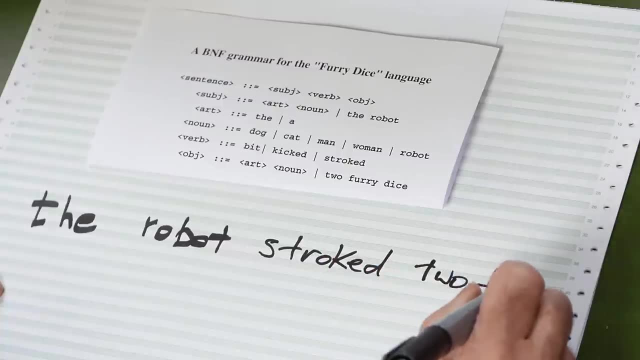 leaves to the root. So, in fact, let's write that test sentence below here. The robot stroked to furry And actually, since layout doesn't matter too much at the moment, I'll squeeze the word dice in at the right there. Now be clear. we're talking about bottom-up parsing. now, In bottom-up parsing, you. 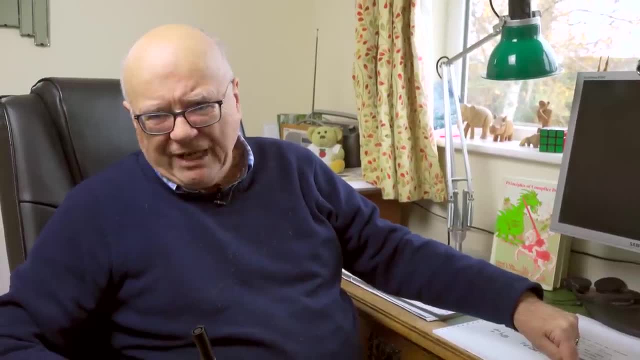 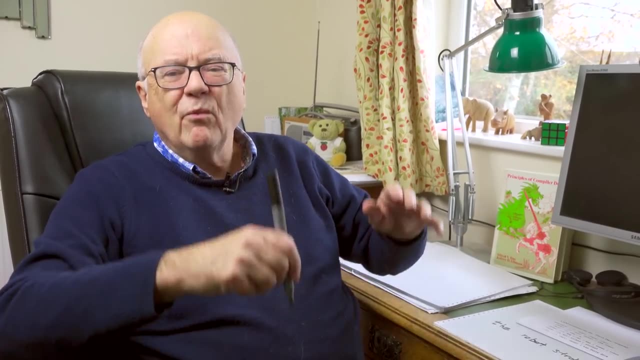 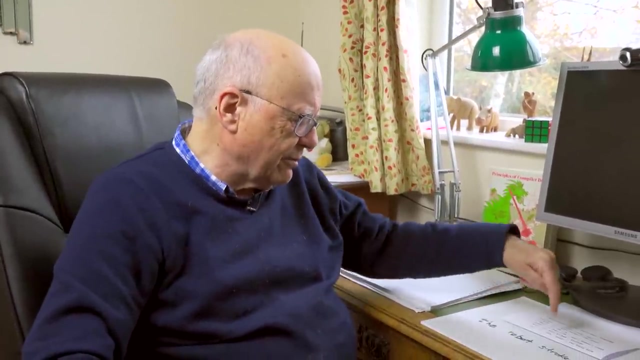 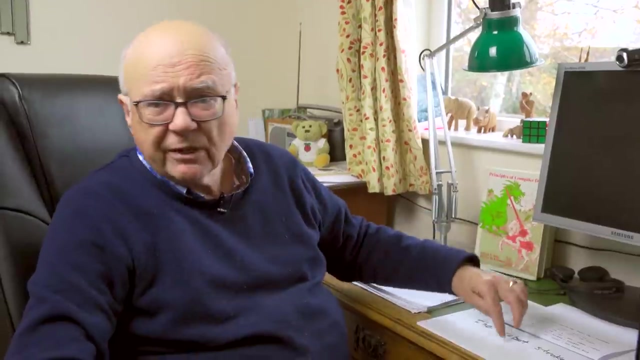 start with the string that you think is correct. and you say: start with a string. can I look into the rules and see how to work up the tree, not down the tree? And yes, so therefore you're looking at possible matches on the right-hand side for components of this string. reading from left to right: 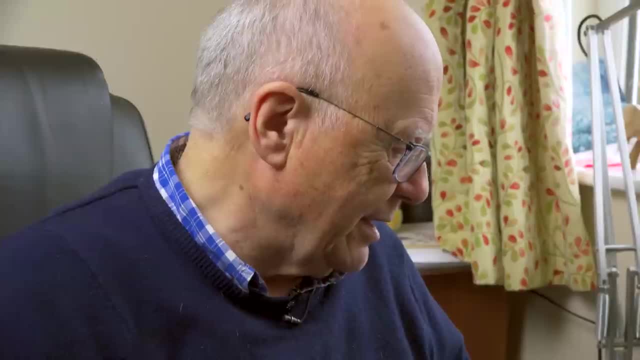 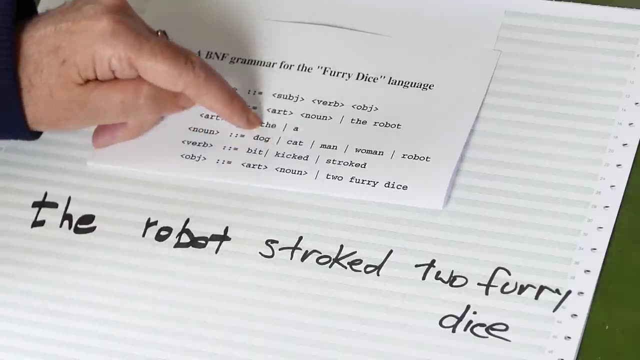 OK, The. How many ways are there? you can match the string the against one of these classifications here. Well, the text, the string the is the right-hand side possibility of an article. That's one way to do it. Oh, and then look up here, right. 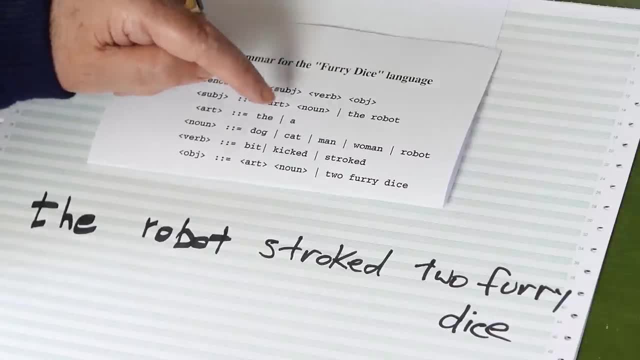 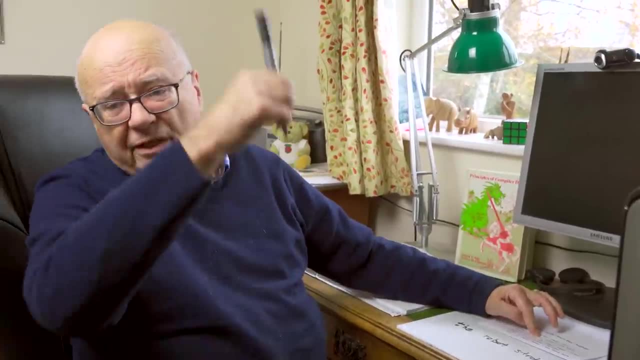 at the top of the grammar. If you have an article followed by a noun like the, followed by something else, that could be a subject and that's looking good, because right up at the top of the grammar we want to end up with subject, verb, object. Looking just at the 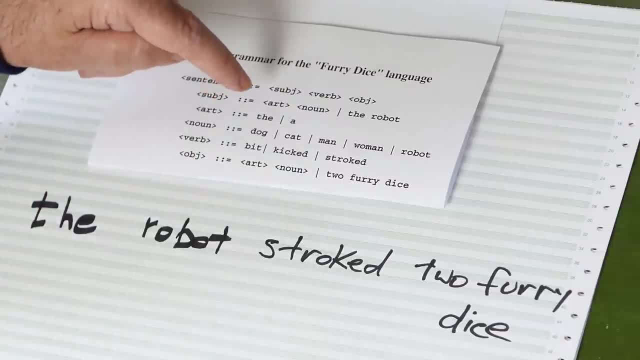 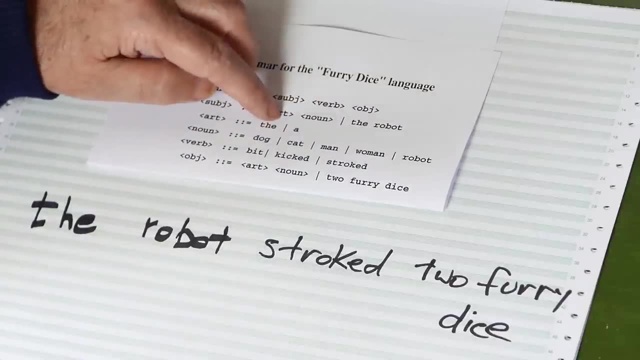 robot. and looking at the grammar right-hand sides, I could do it by saying: well, it's the subject of the sentence, it's at the left-hand side and if I go article noun, I get the and I get robot. But what I've done, just to act as a 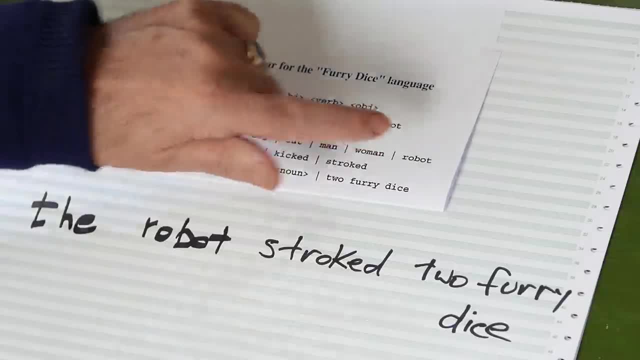 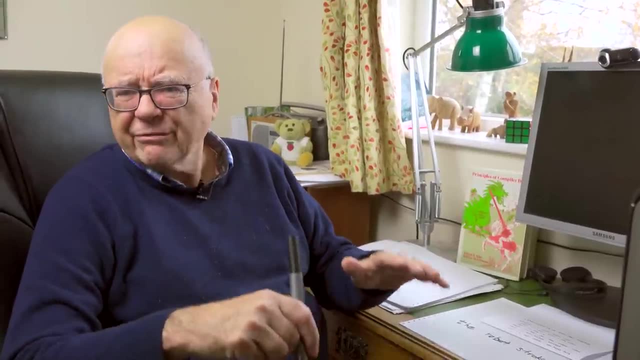 talking point and it illustrates a lot of things. here I've given you a shortcut. If you want to, you can just do the robot with no further interior analysis at all. It's an allowed phrase, It's the subject. Now I have to say that, as we 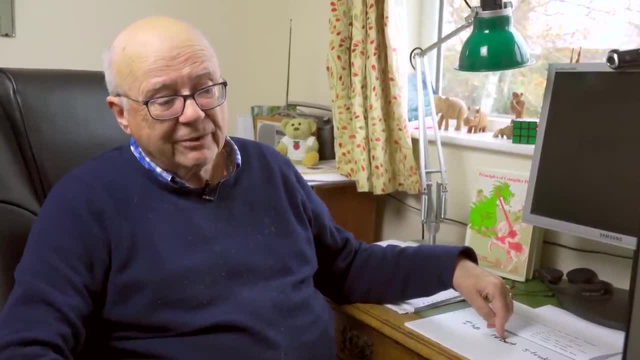 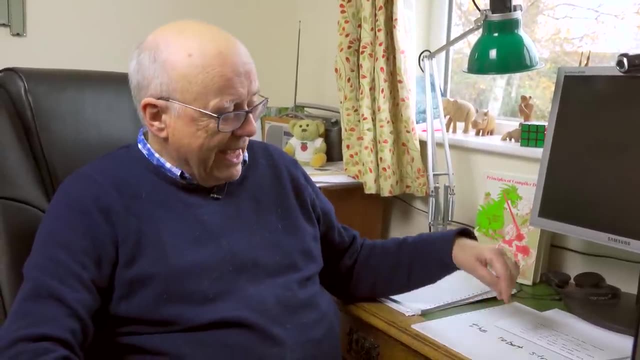 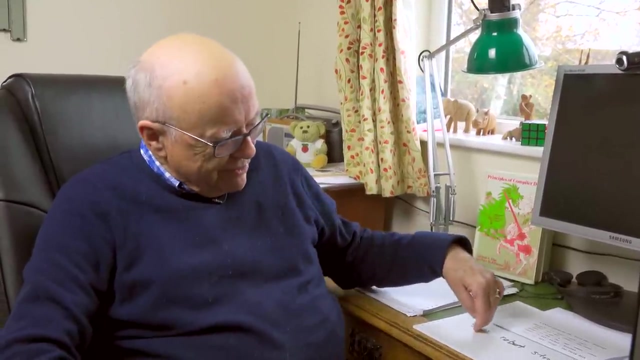 develop this story. we will get into bottom-up parsing, because one of the tools we're going to use, called YAK, basically produces bottom-up parsers for you, not top-down ones, And it's a YAK behavior symptom that it loves when you're trying to match text strings, It likes to match the longest one that it. 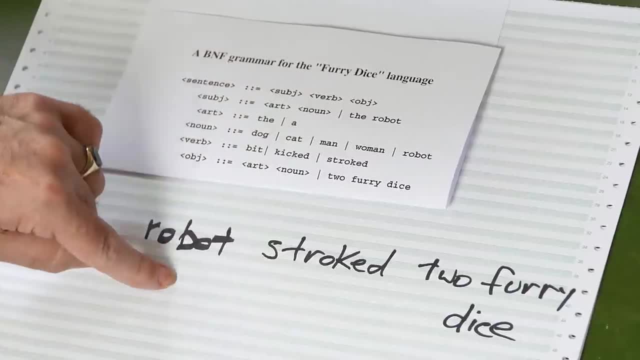 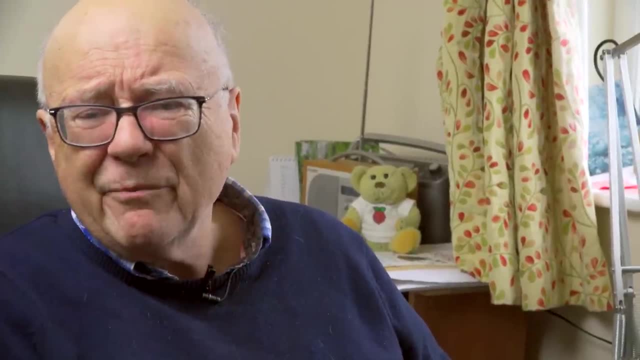 can manage. So it is going to seize on the robot all as one phrase, as being a wonderful long solution. Why doesn't it just do the and then wait patiently for noun? That's not the bottom-up way. If you can see a longer Oh, and this thing by. 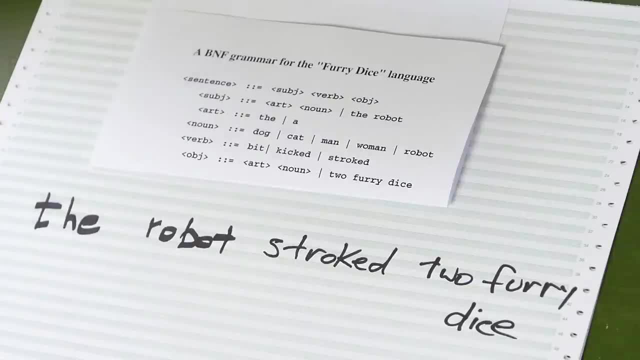 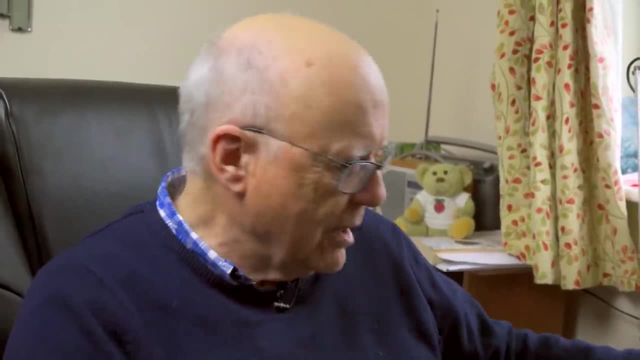 the way that you're looking at is built upon a stack. of course, It's called the handle. I get a longer handle by going for this option here And getting the robot all in one go. Okay, the robot, then, And you've got to get. 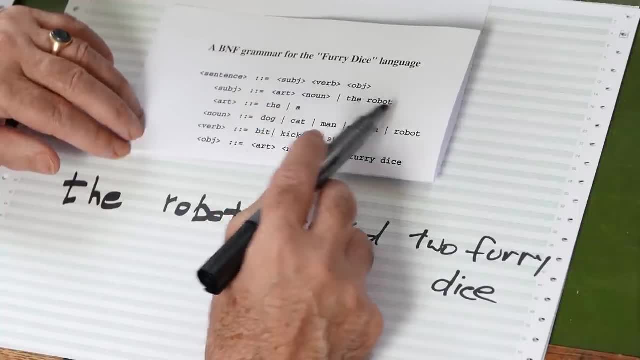 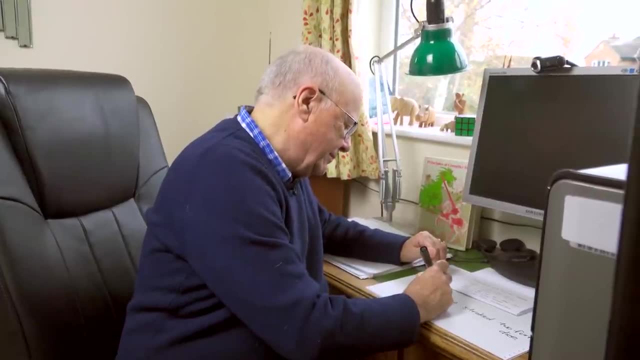 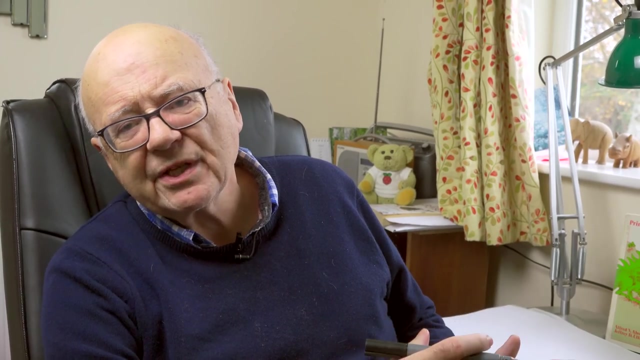 used to reading from right to left, now in bottom-up, parsing The robot all as one phrase, is an example of a subject. So we can now say: okay, the robot is my subject. Now that act of picking up a substring from your sentence and going 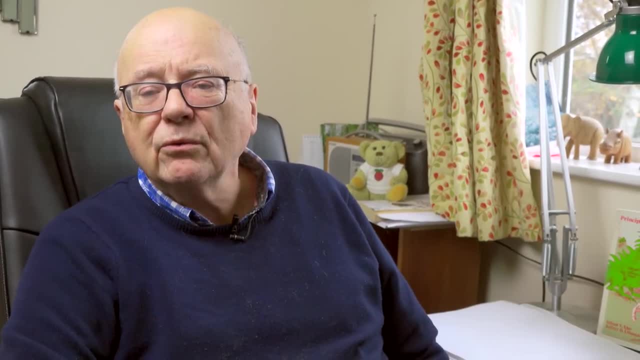 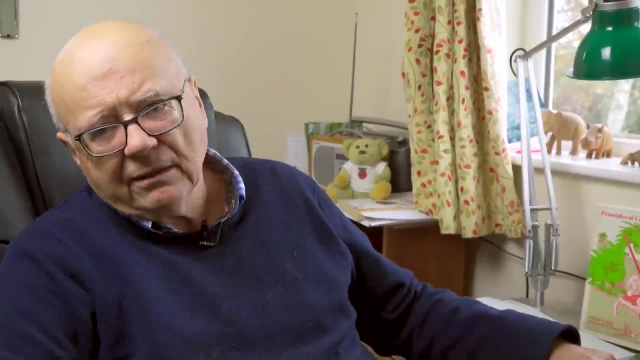 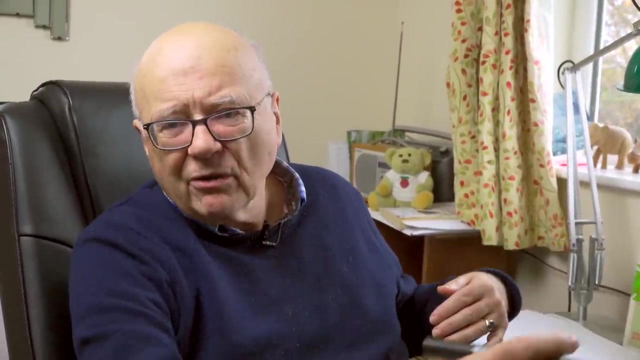 upwards and making it more abstract, if you like, is called reducing in bottom-up parsing, So looking for a longer and longer and longer string to get your handle. That's called shifting, because you're shifting characters one after another and making the string longer and longer and saying: can I go any further? That's shifting. But 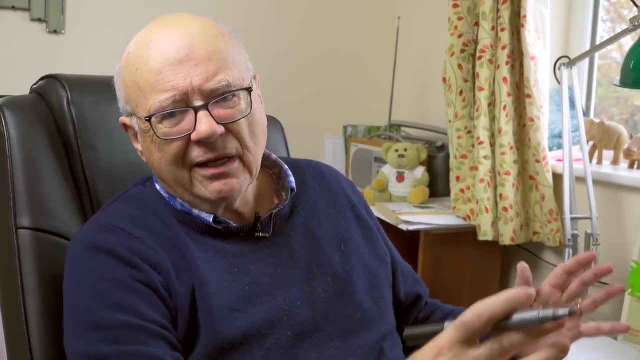 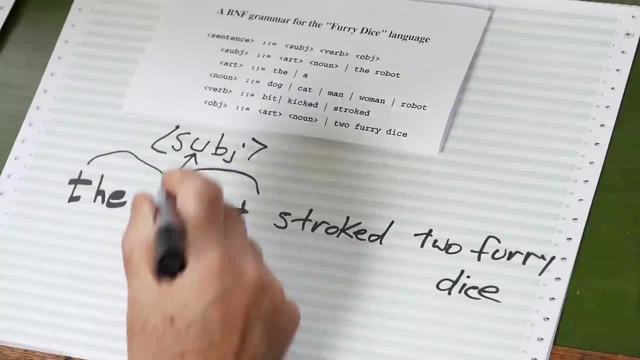 when you say, oh, that's a nice long string and it matches. and then you go up and say, oh, that's my subject. that is called reduction, because you're going to something simpler further up the tree, So you can tick that off as being done. 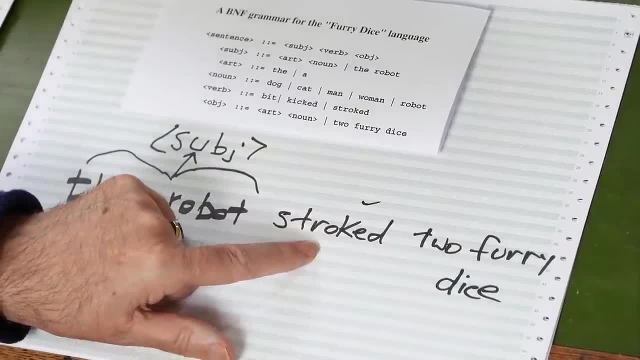 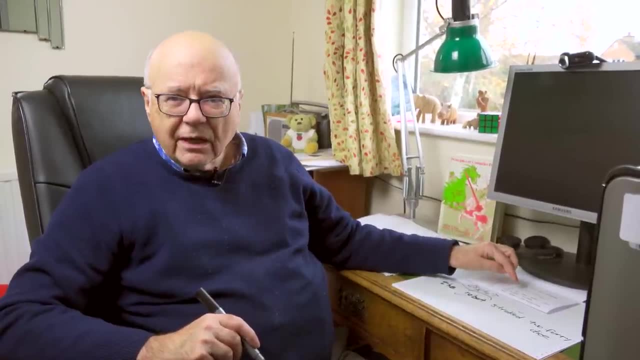 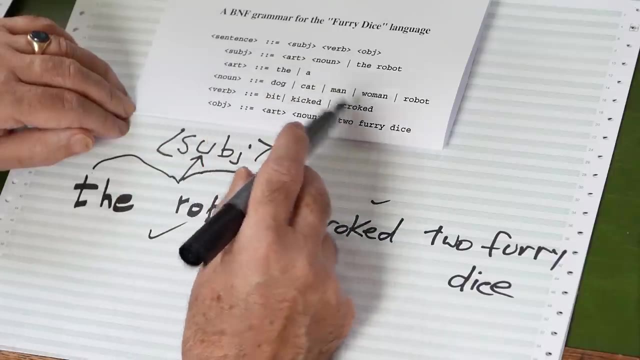 bottom-up. Next thing is you see this string of characters called stroked, And once again it's right-hand side driven. What is there on the right-hand side and which rule is it that could possibly match stroked? You're seeing here, against verb bit, kicked or stroked, Those three. 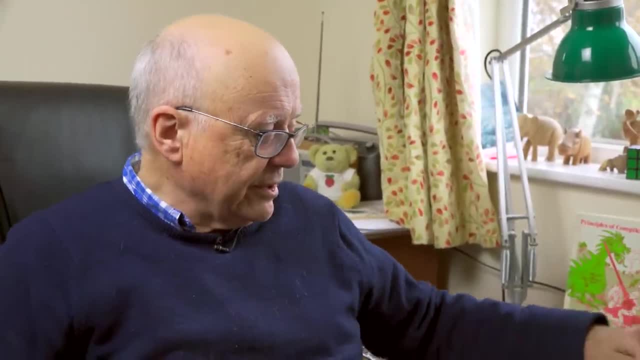 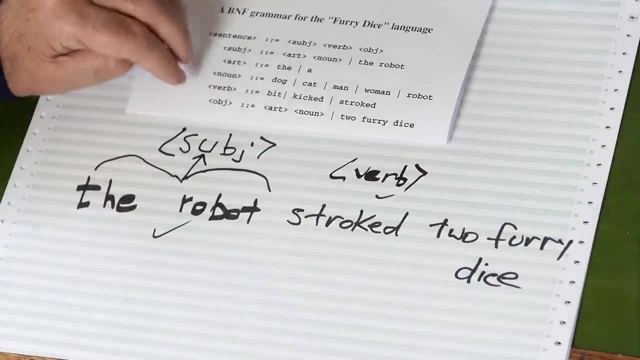 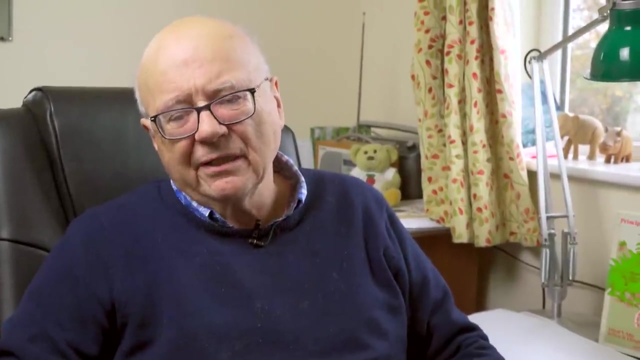 strings are your possibilities, So that's fine. Going right to left, you say stroked is an example of a verb. So we've got our verb there Now again cheated, but it's wonderful fun. I have not analyzed two furry dice into adjectives and nouns and things like that. 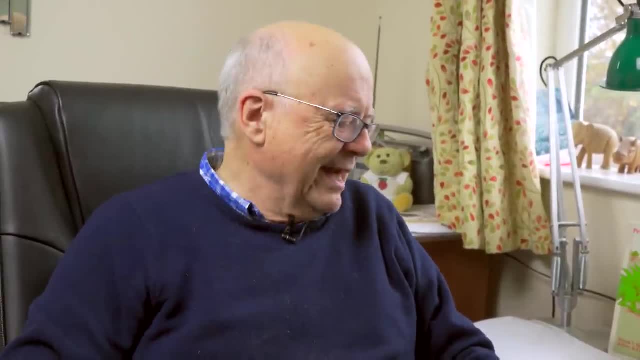 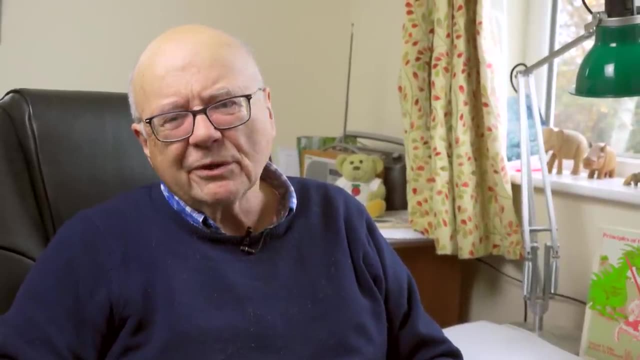 I've just put it in as an interesting shortcut to have there, And it is an example of what I would call an object phrase. Some of you who are really good English linguists may want to go on about my lack of understanding about what a direct and indirect object are, not to mention predicates and so on. But 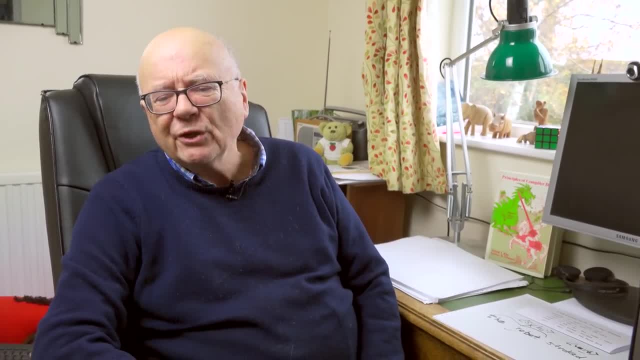 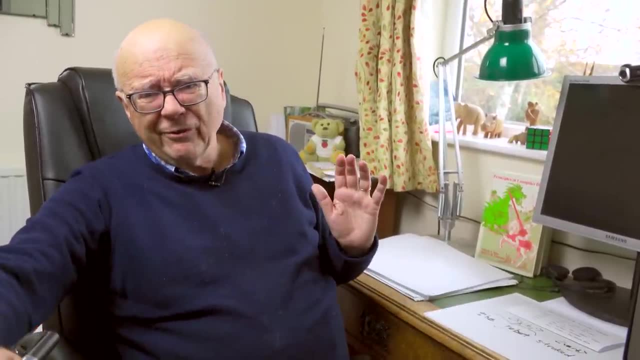 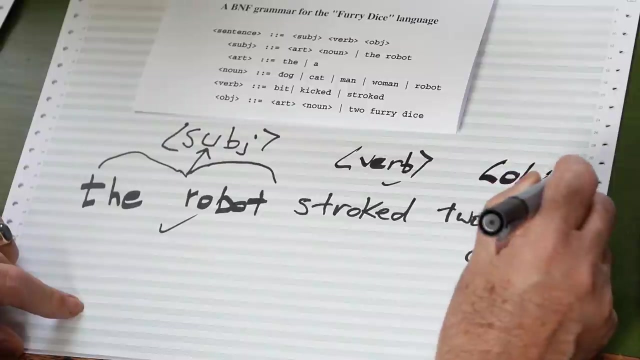 please forgive me, I regard it as being a phrase in an object position. So I'm saying: there's a quick match here And bottom-up is going to love this. Two furry dice, a great long handle. Oh, and if I match it there, what's the left-hand side? it corresponds to Obj. Okay, then we've won. 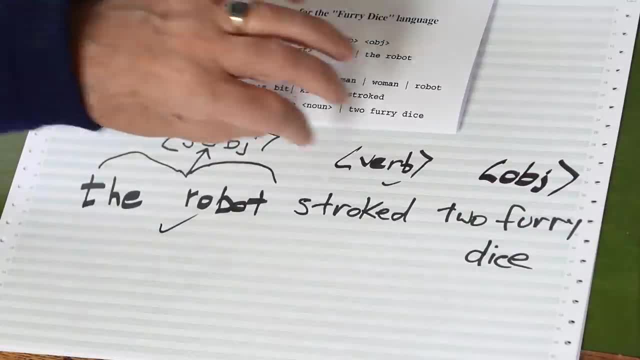 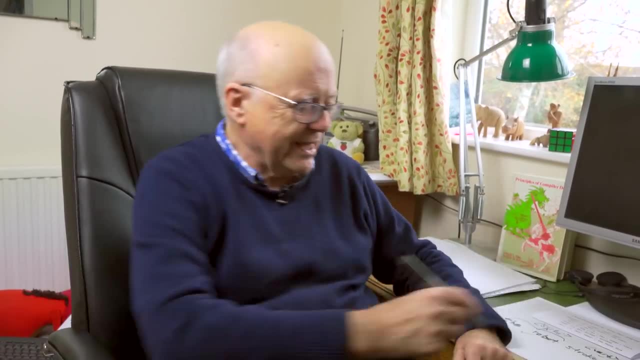 We have worked bottom-up to having subject, verb, object on our stack, starting with the string, And, what's more, we've exhausted the string. now It's the end of it, There's a sort of full stop after that. There we are, then We've got. 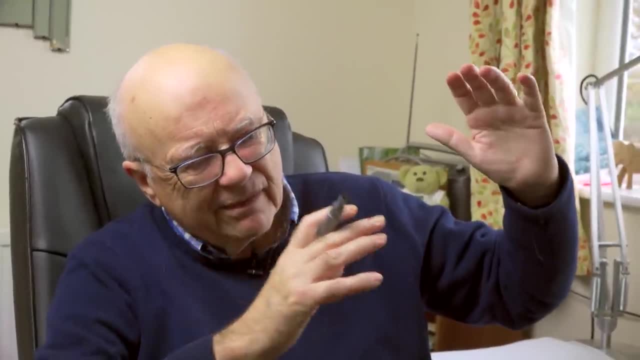 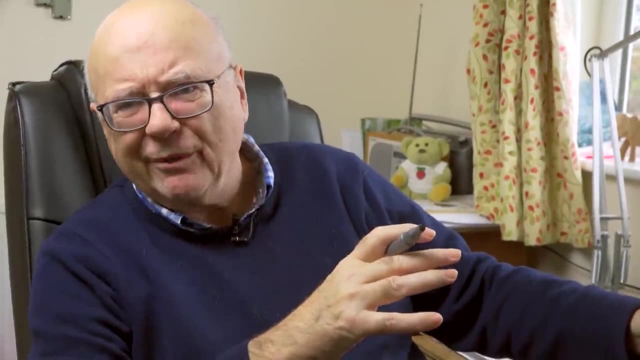 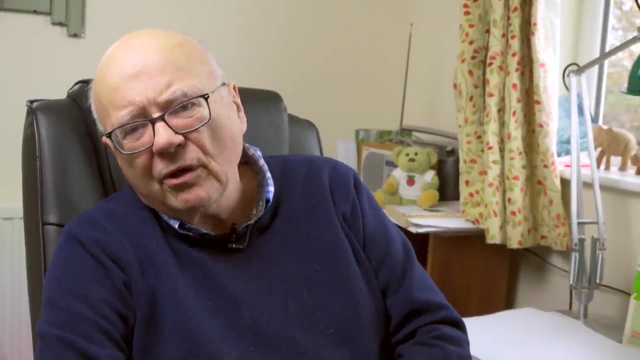 top-down, which tends to be more- how shall we say- Eager. You know, a top-down parse would very probably leap on the word the and not bother to go any further because it's found a quick match for it, Whereas bottom-up is the other way round. It's basically saying: I want the longest. 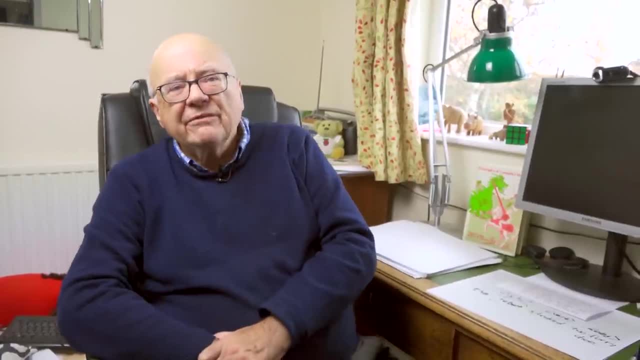 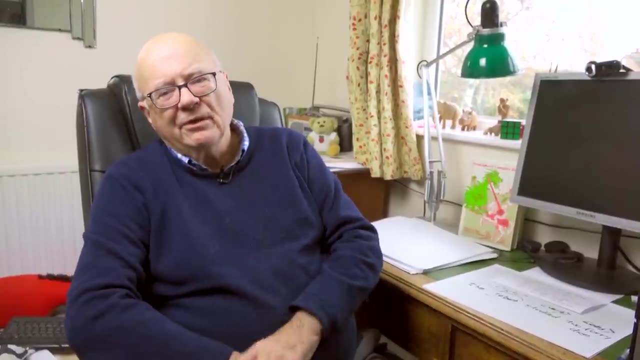 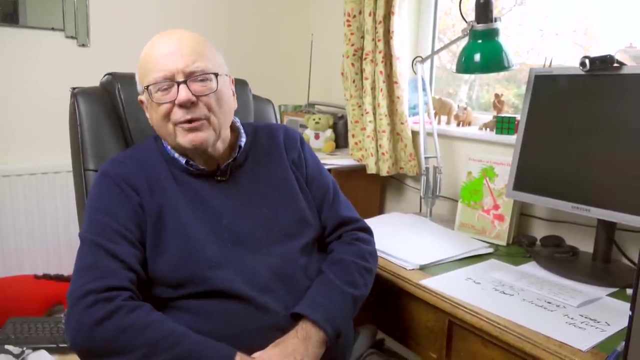 possible handle. Even at this stage in the late 50s and early 60s, there was a sneaky suspicion coming around that actually bottom-up parsing was a little bit more powerful than top-down. I'm going to put out a set of notes for this so that you can look up for. 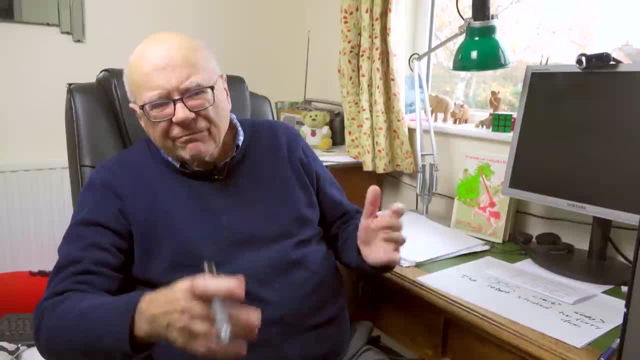 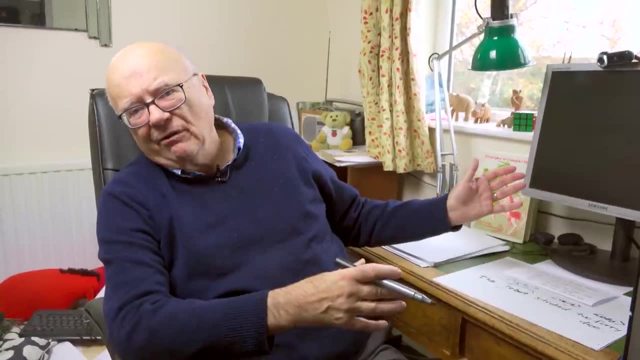 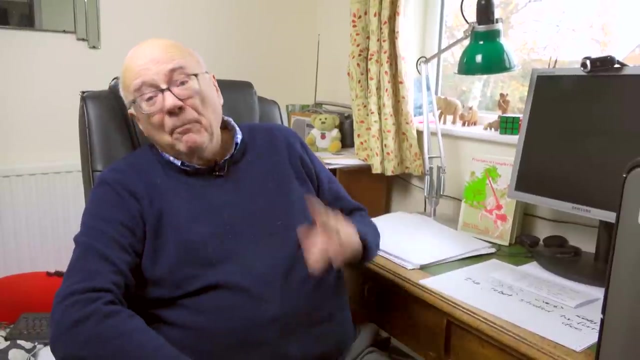 yourself just examples of why it is more powerful. But, roughly speaking, I think you can sense that because you've not only got something you're looking for, but you've got a handle that you've already accumulated. it's like gathering more contextual information going bottom-up But, on the other hand, handling 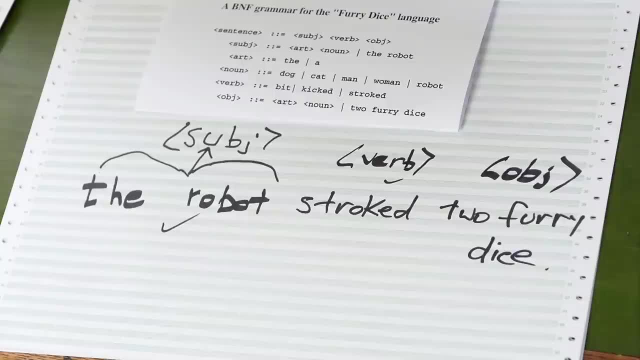 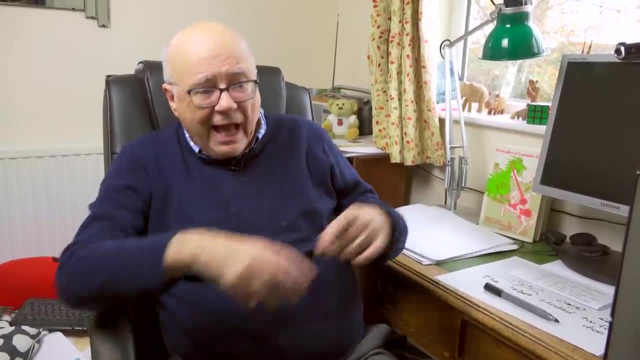 the stack and working out what's happening is a darn sight more complicated if you do it by hand, coming bottom-up. Rather than do it all by hand, why not me and you lot? It's a good way to learn Lex and Yak. In other words, don't. 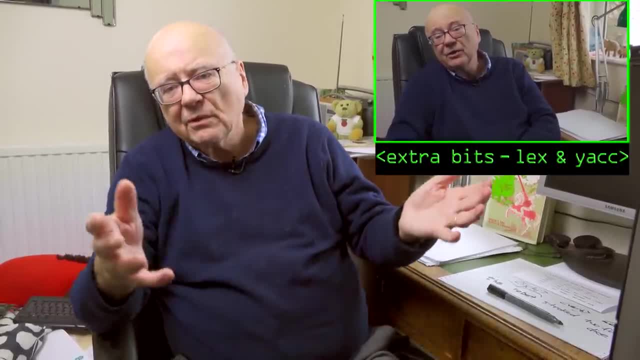 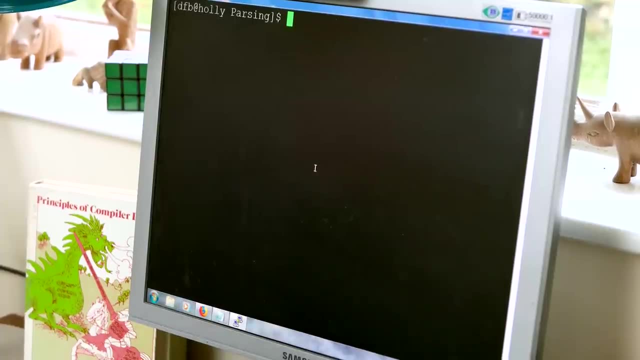 write the C directly yourself. Get a software tool of these like these two to do it for you. So that's exactly what we're going to do. I've got the program Putty that does SSH connected. here I'm talking to my other Linux machine in the. 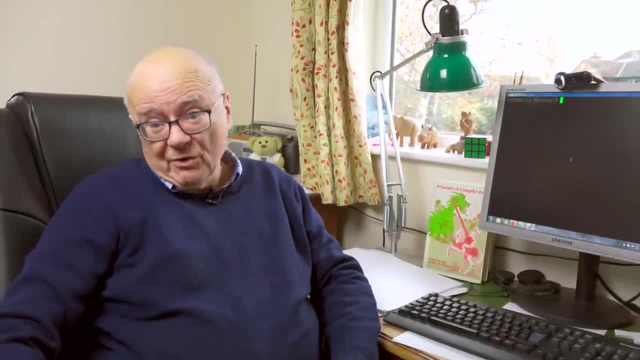 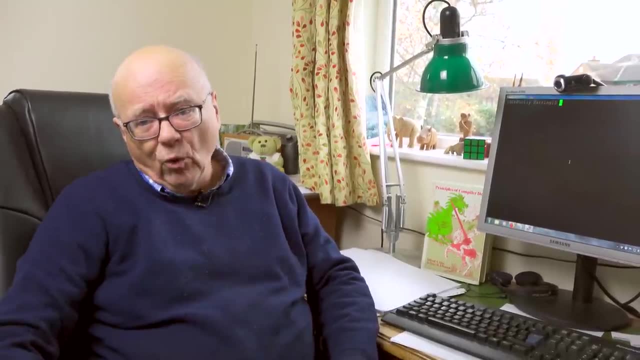 other room where I have got set up a parser, Complete parser, Front-end, Let's Call Analyzer. We're going to do a syntax analysis for this furry grammar and all legal sentences in it, And I know first of all you will want me to call up the program. 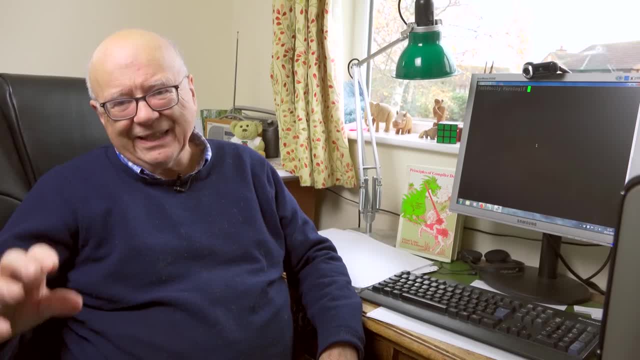 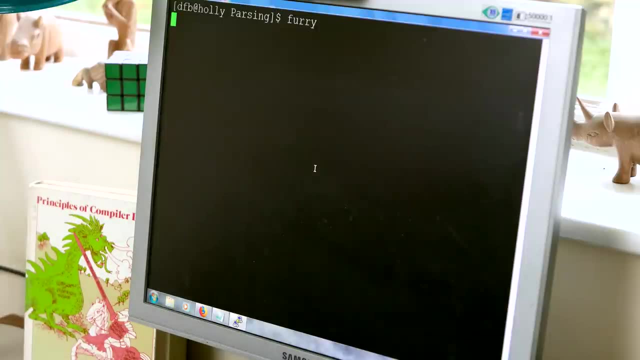 that implements this, And the test sentence first of all is the robot's throat to furry dice. Here we go, So furry, It's hanging there, It's waiting for us to give a correct furry sentence. Dice return. Look at that. 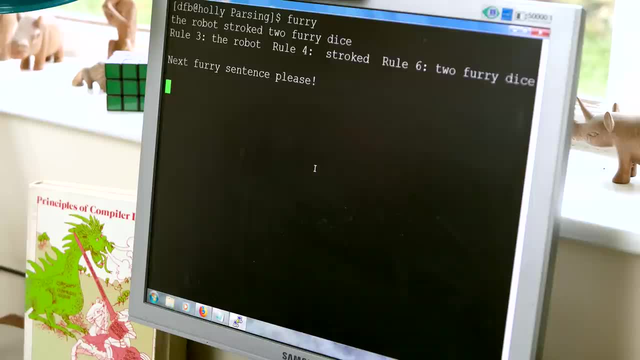 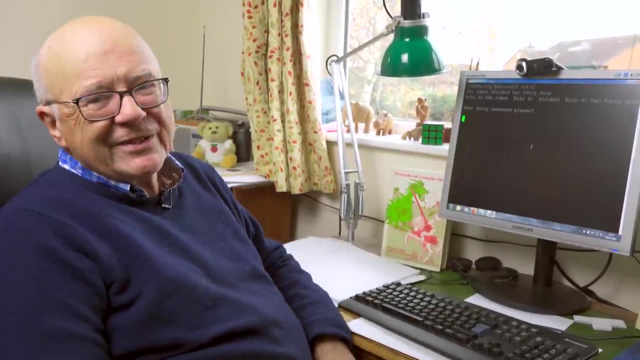 I'm happy with it. I've given it in subject, verb, object order, And I have numbered those rules in the grammar, as I showed you earlier, And I now have, as it were, a map of how it has parsed it. Rule 3. Now, that is the one that effectively. 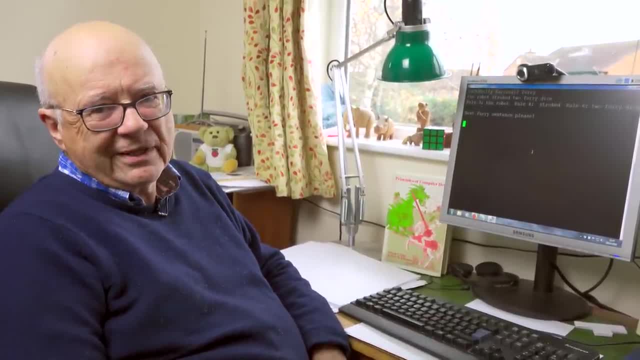 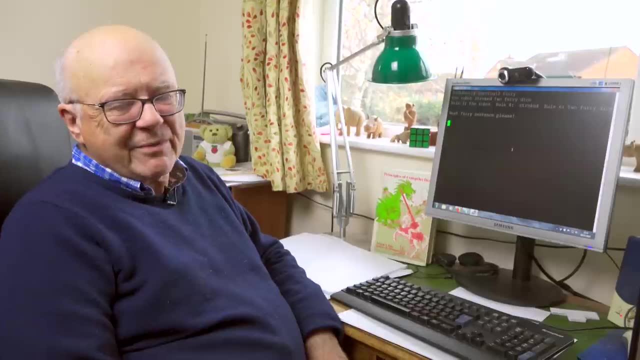 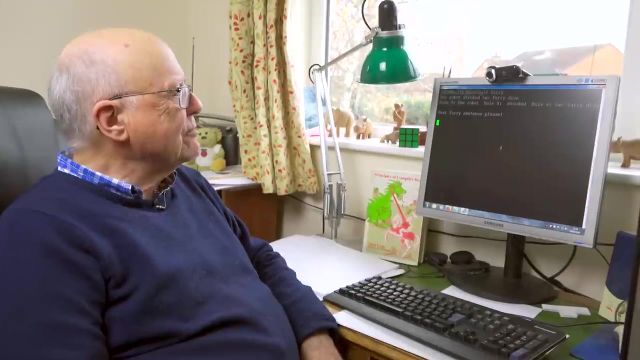 says I can do the robot all as one phrase. It has chosen not to go for the and robot as article and noun as separate entities. It might well have done that had I gone top-down, But because this yak-confected parser system goes. 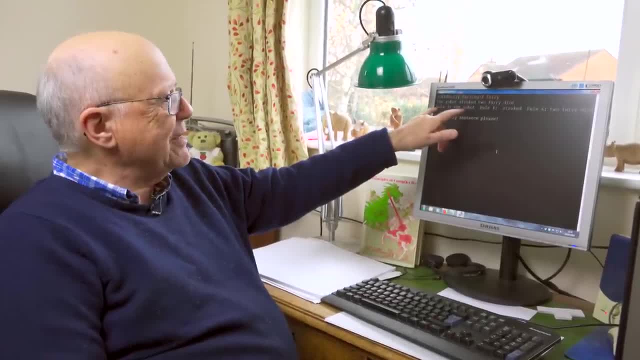 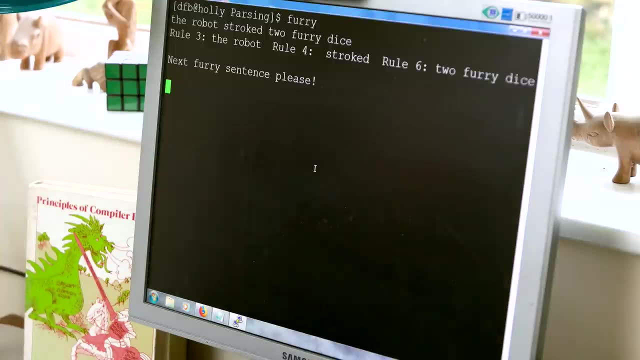 bottom-up. it's gone for the longest possible handle at that stage And it's matched it Rule 4.. The middle piece is matched, stroked as the verb And finally it is spotted right at the very end that I've put in another sneaky shortcut Two. 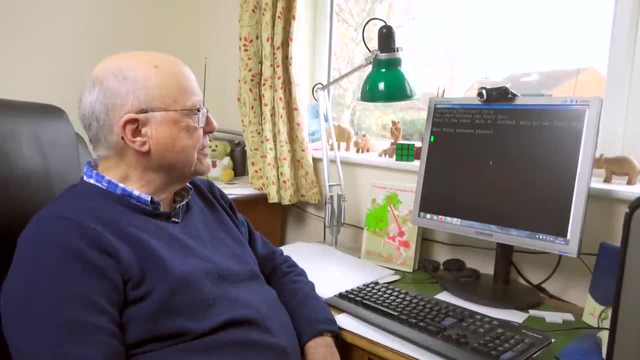 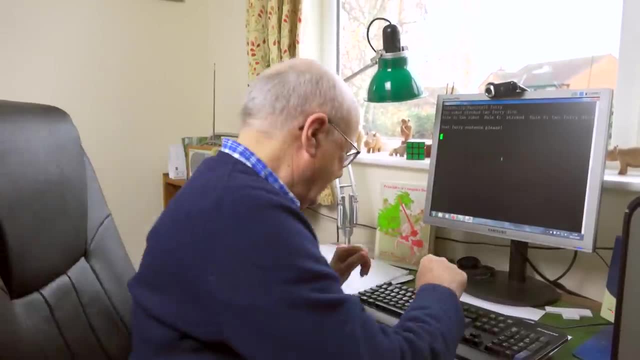 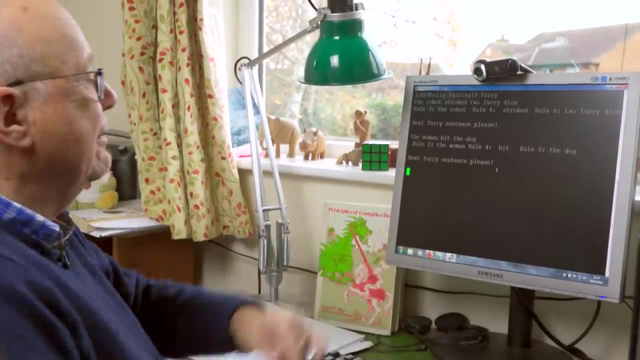 furry dices. Rule 6. And that is my pars, So shall we try one more? Just to make sure? Go on, Sean, Tell me which one to try. The woman bit the dog. Yep, The woman bit the dog. There you are, Look. Rule 2. The woman. 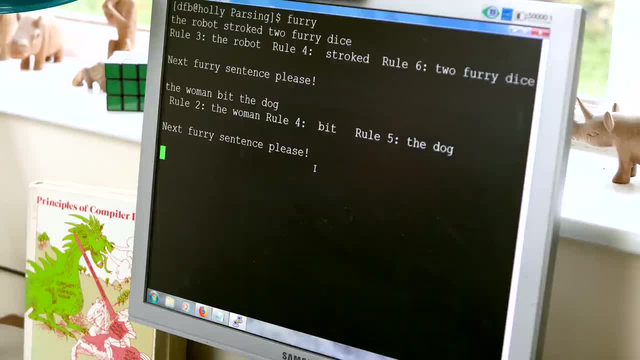 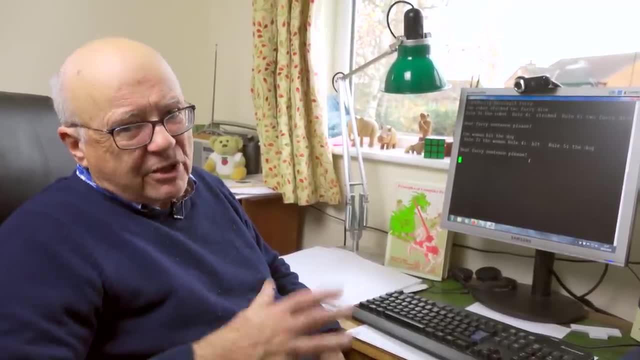 Now rule 2, not rule 3.. If it's followed rule 2, it's gone down the article noun route, Which means it knows that's the only way to match the woman. There is no shortcut way. Okay, Rule 4.. Verb Rule again. It chose bit, Rule 5.. Now 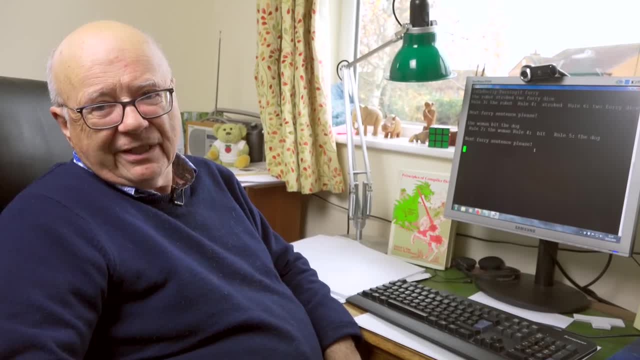 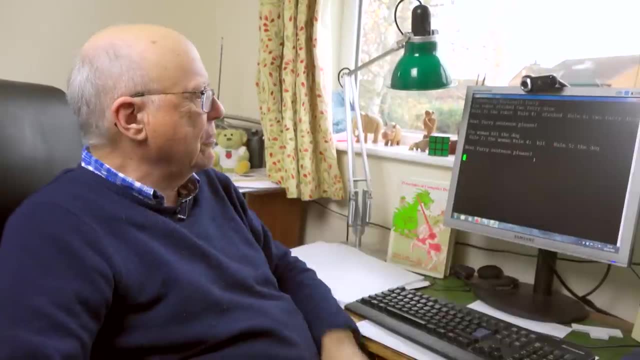 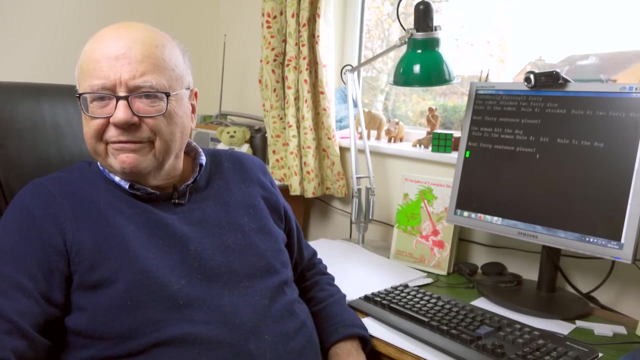 this time again, there is no shortcut to two furry dice at rule 6.. You've got to go the long way around And, following rule 5, you break it down into article noun again: The and dog. So there we are, We. You could say: well, you've written a compiler for the furry language with the. 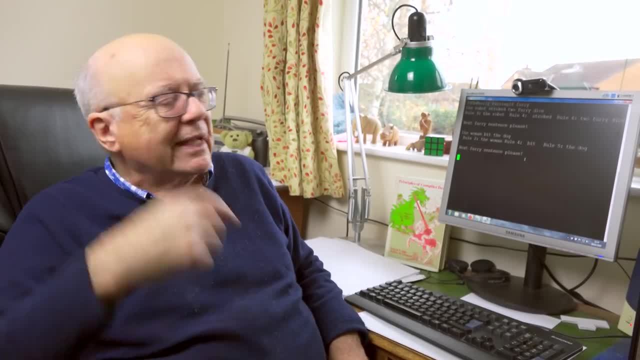 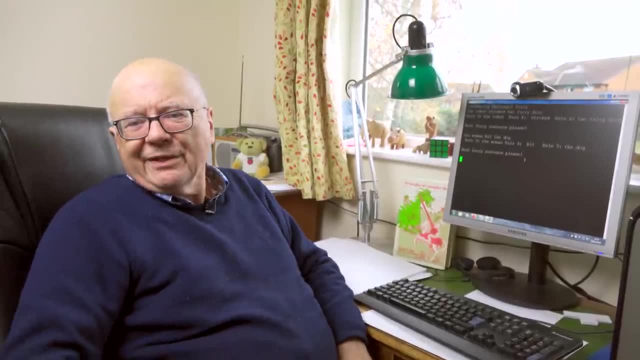 help of Lex and Yak. We can go into details of that later if need be, But not now. It's fair enough, But it's not doing anything, really, is it? What more should we do with this now? We've written it this far, then, Sean, You tell me. Well, I think next time we need to do this.